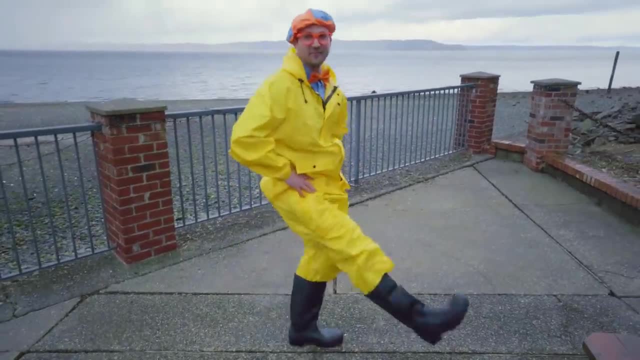 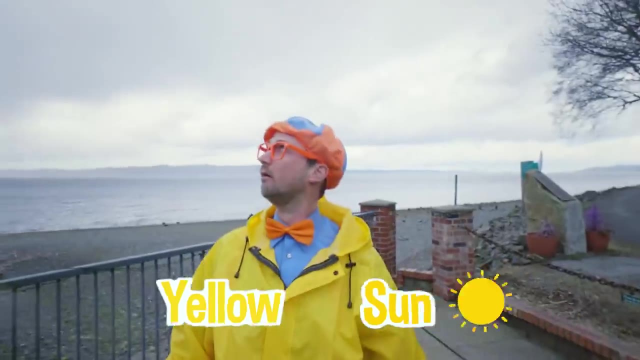 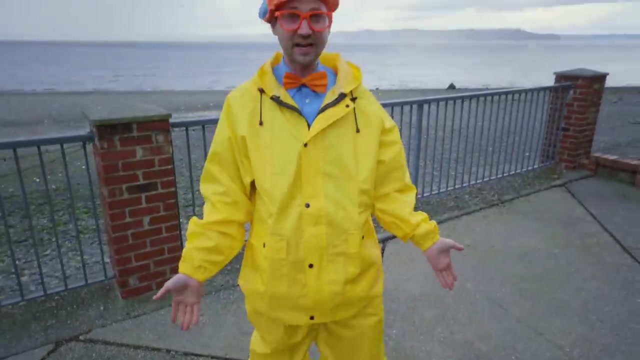 And I got my matching bottoms on. Yeah, What color's my outfit? Yeah, It's the color yellow, just like the sun. Where's the sun, I don't know. But hey, check out my boots. Yeah, I have black rubber boots on. 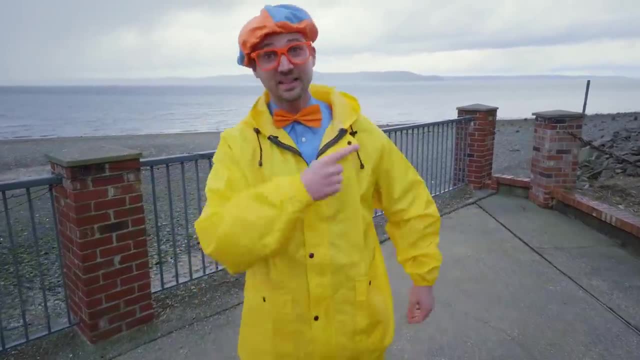 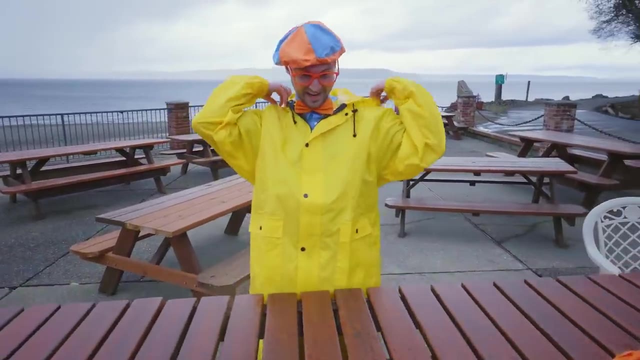 And the last thing that I'm missing. yeah, let's go find an umbrella, Whoa-ho-ho-ho-ho. Okay, let me put my hood on. Wow, it's really starting to rain. All right, check it out. 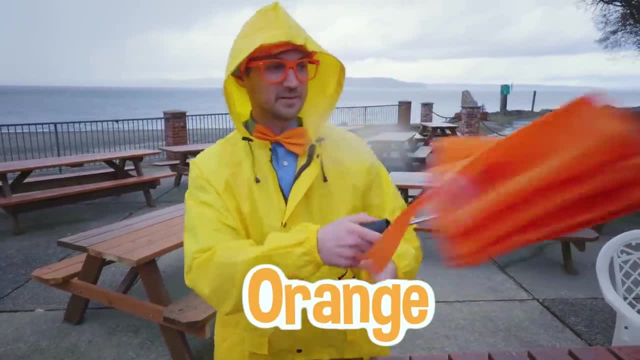 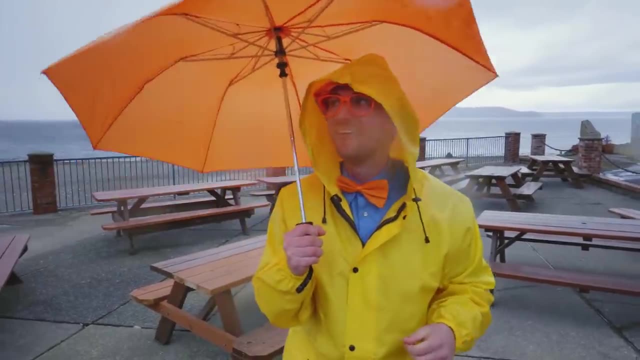 An orange umbrella. Let's open it up. Whoa-ho-ho-ho, Whoa-ho-ho-ho. Now there's no rain hitting me at all. Whoa, Okay, let's put this one away. What's this next one? 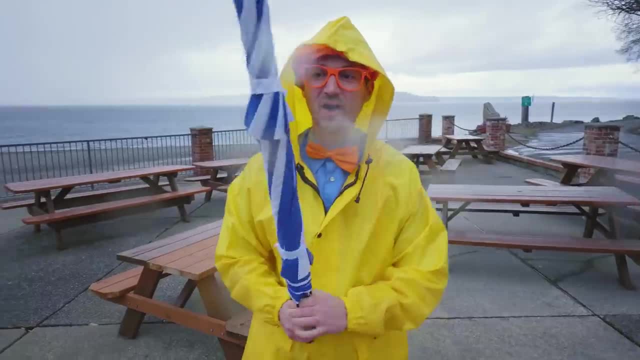 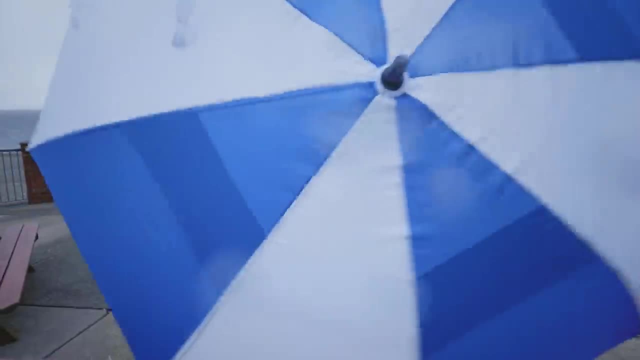 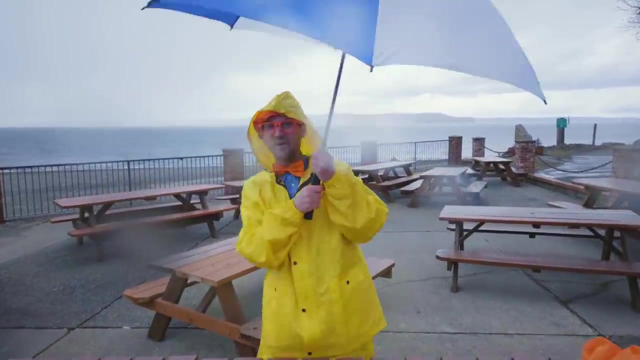 What's this one? This umbrella was really small And this one, whoa, is so big. Whoa-ho-ho-ho-ho, Whoa, check it out, Whoa-ho-ho-ho, What color is this umbrella? 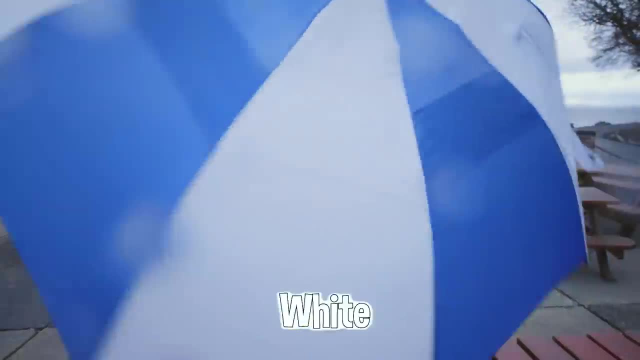 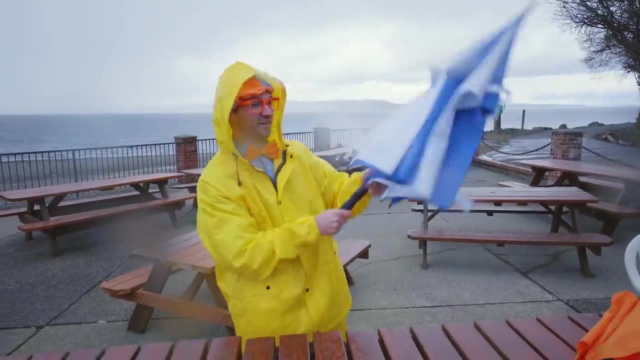 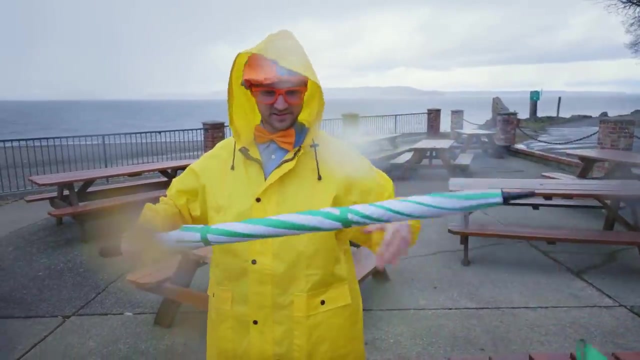 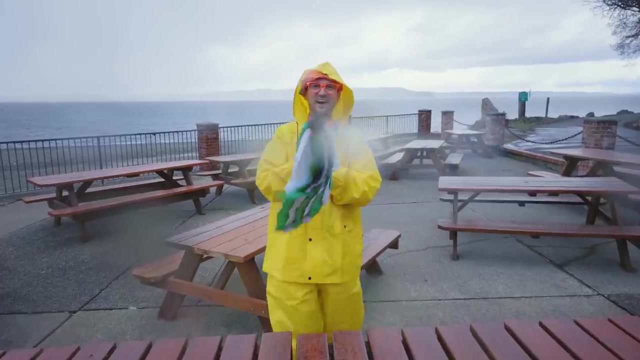 Yeah, Blue and white, Whoa-ho-ho-ho. Okay, let me put this down before I fly away. Okay, And for this umbrella: whoa, check it out. Yeah, another big umbrella, And the colors of this umbrella are: whoa, it is so stormy out. 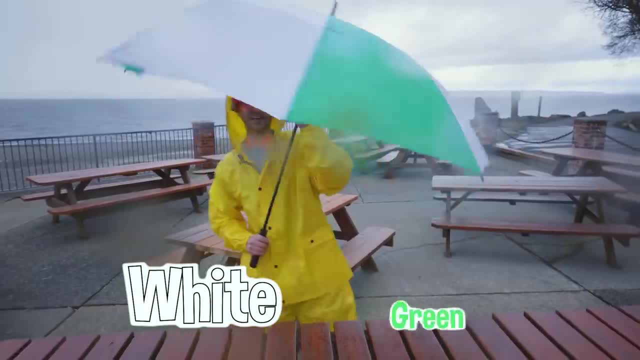 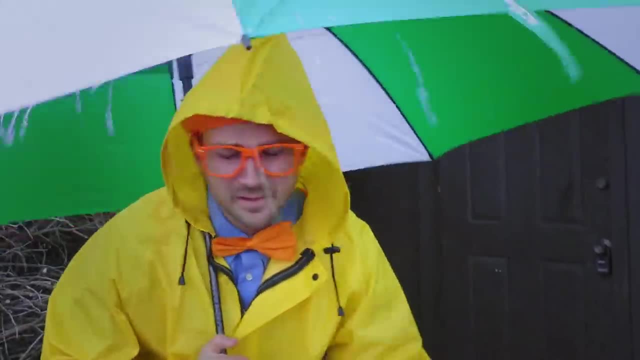 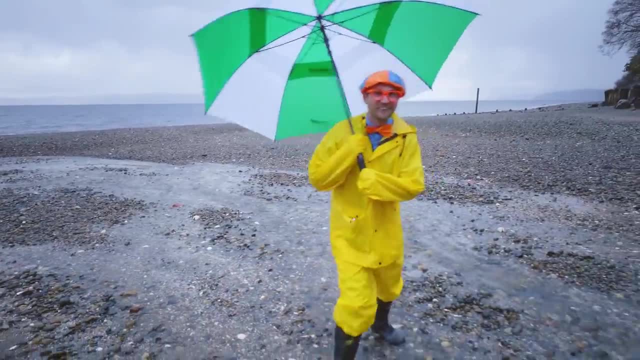 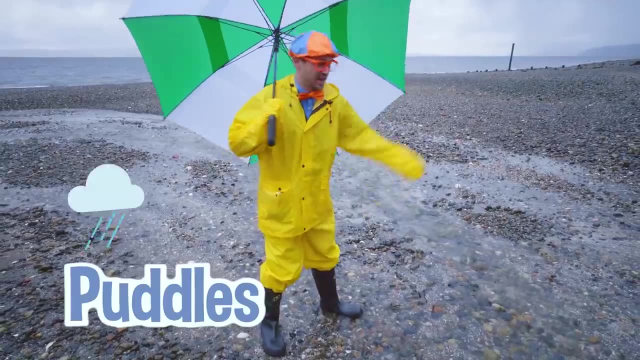 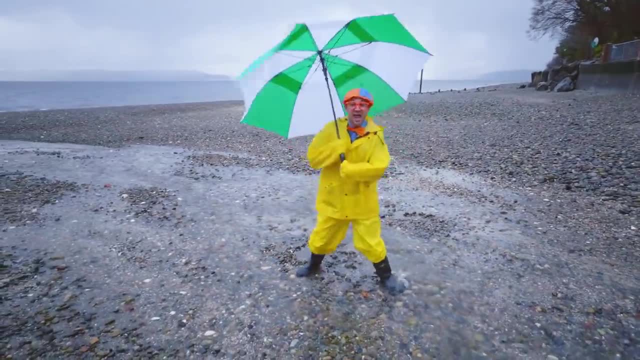 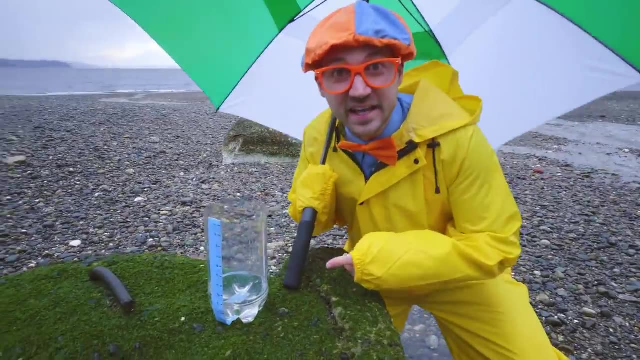 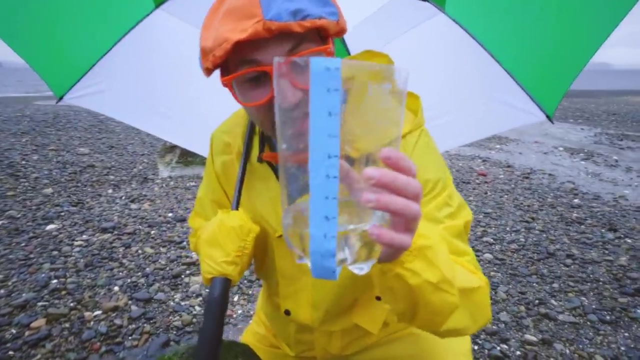 Woo, Woo, Woohoo, Yeah, Yeah, Look back here. Wow, Do you see this? Yeah, this is my rain collector. I set this out earlier, before it started to rain, And then all this rain collected from the top. 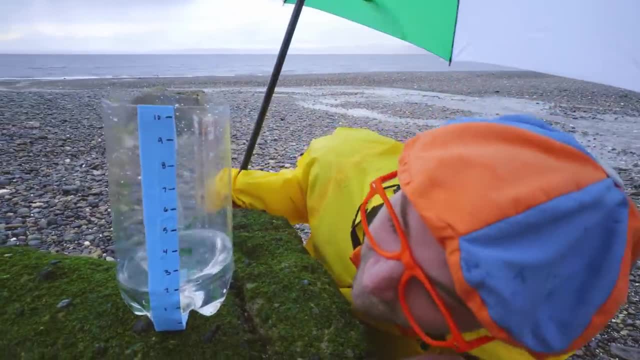 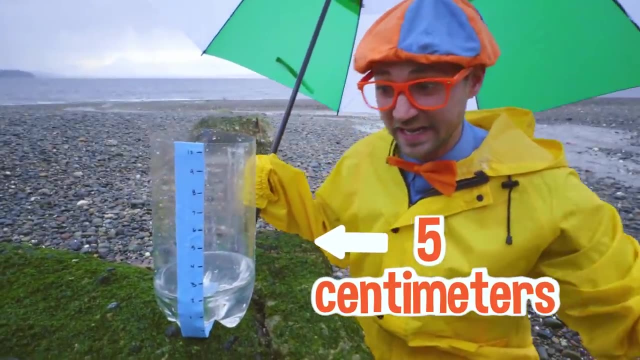 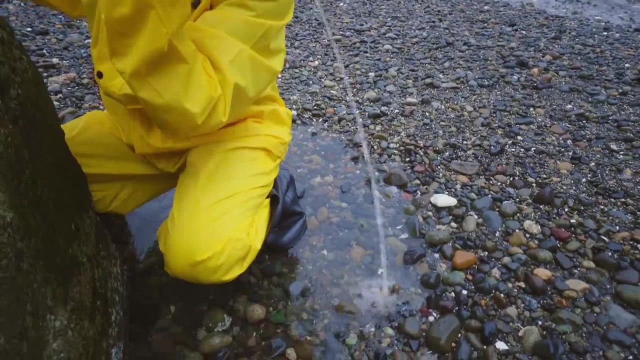 Do you see how much it says Wow? Yeah, it says about two inches. Yeah, that's just over five centimeters of rain. Wow, that's a lot of rain. Okay, I'm going to pour it back onto our planet Earth. 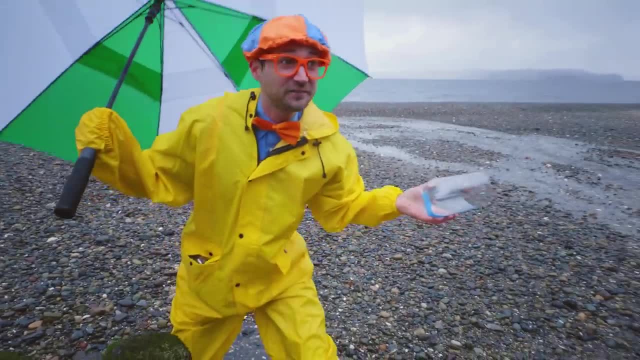 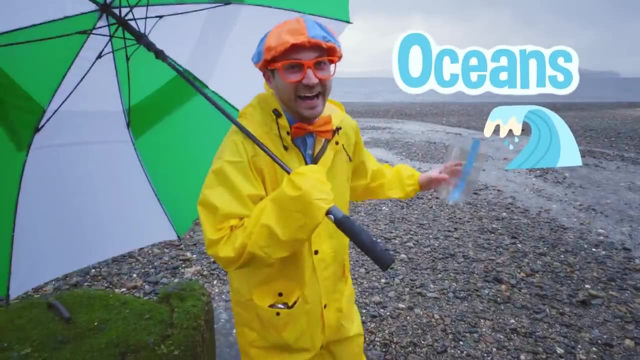 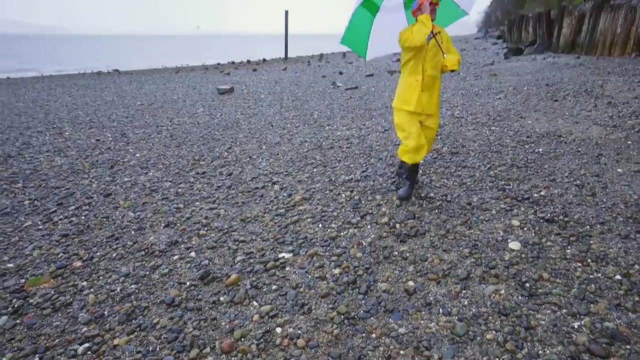 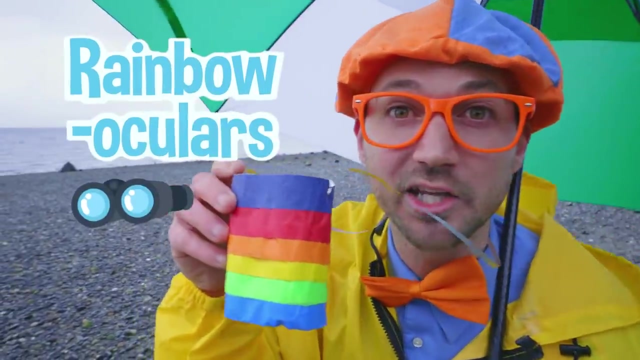 Because when the rain falls on our planet, it's really good for it. It helps keep all the plants nice and moist and our oceans nice and full. Woo-hoo, Woo-hoo, Hey, Hey, Check it out. Yeah, these are my rainbow oculars. 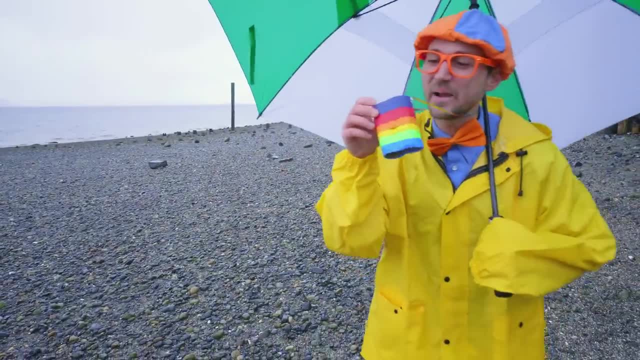 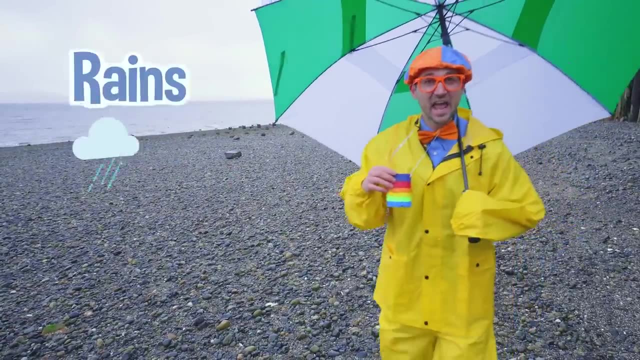 Yeah, isn't that cool. Yeah, they're the colors of the rainbow. Have you ever seen a rainbow before? Yeah, they love to come out after it rained. Yeah, a rainbow is an arch of colors made by light and water. 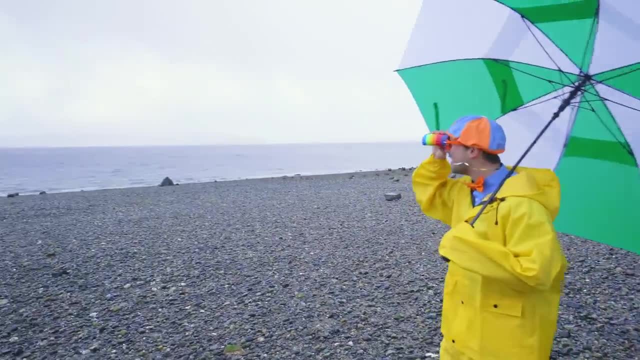 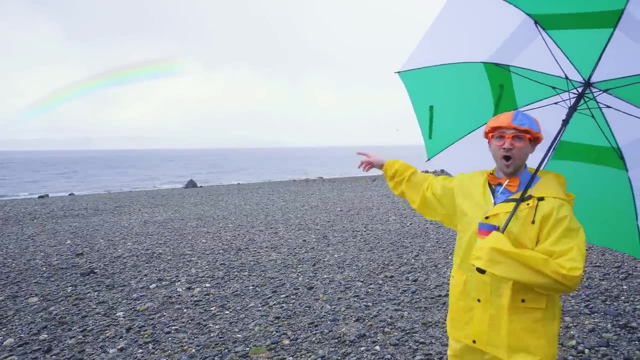 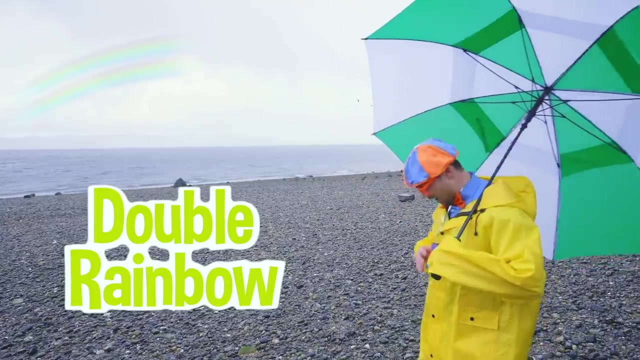 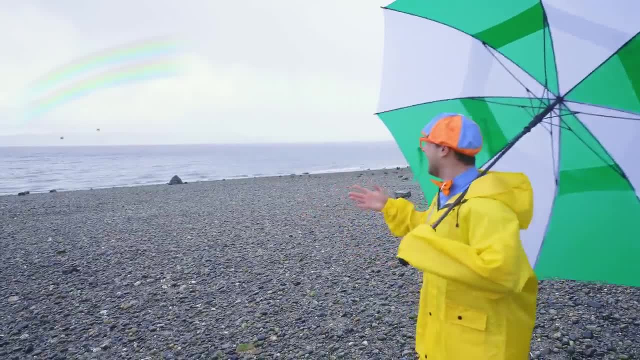 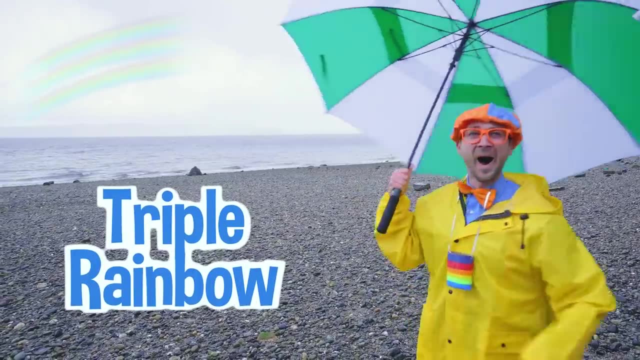 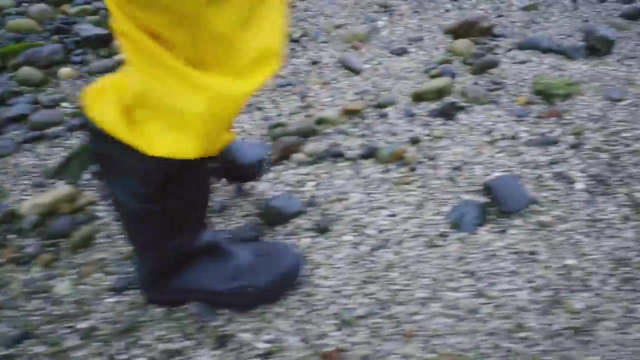 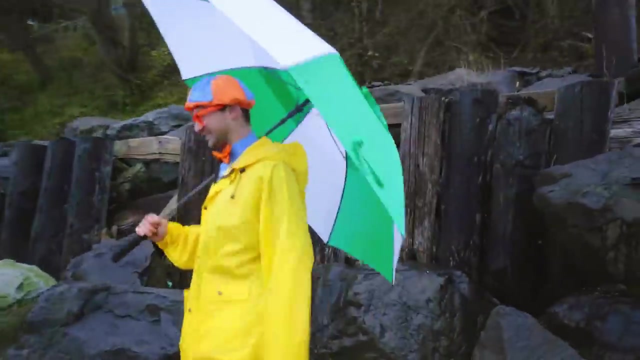 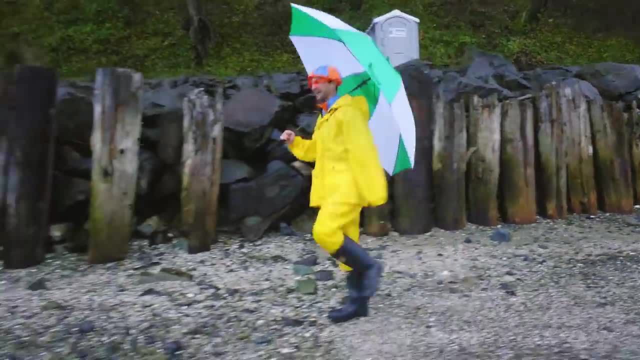 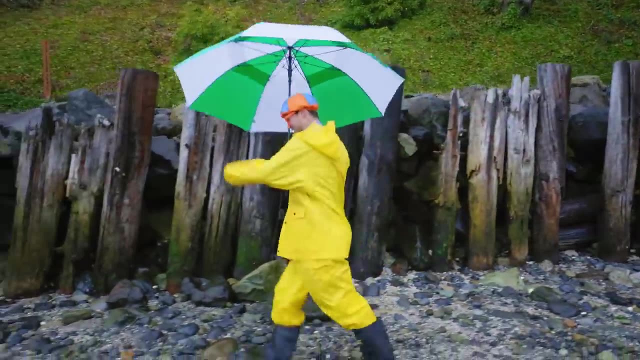 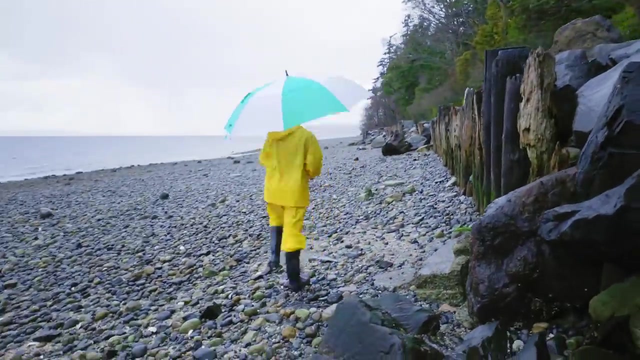 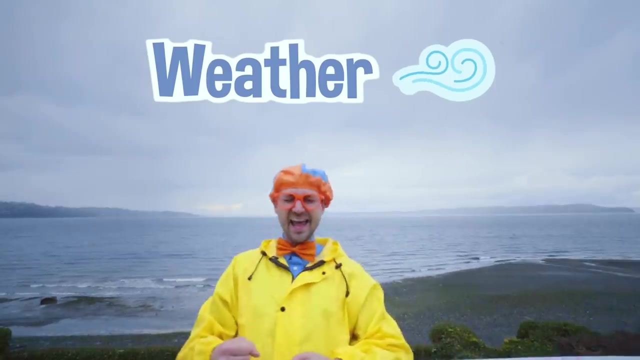 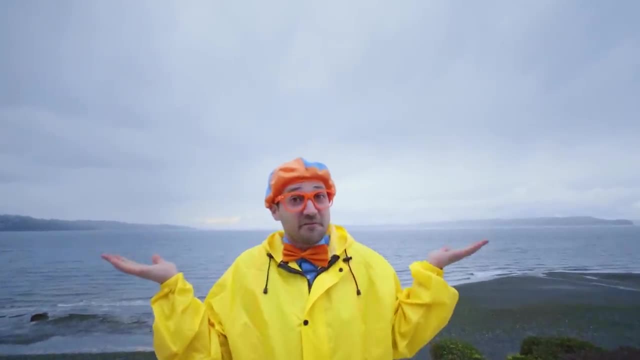 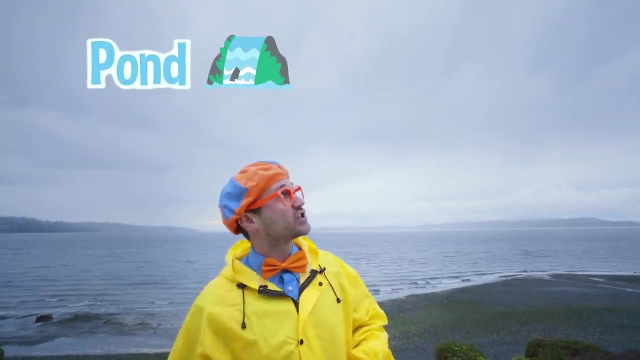 Woo-hoo-hoo-hoo-hoo, This weather has been awesome, Yeah, Hey. have you ever wondered where does rain come from? Well, let me tell you, Haha. Okay, let's start with water in a pond or a stream or the ocean. 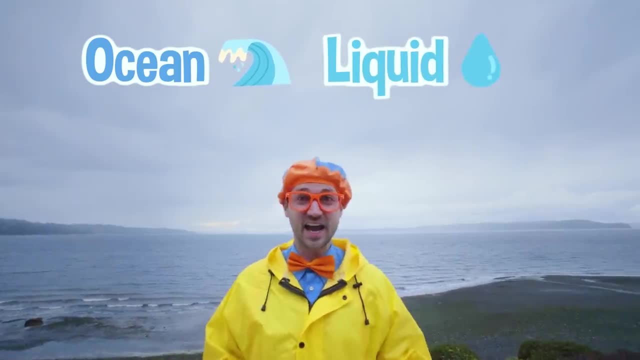 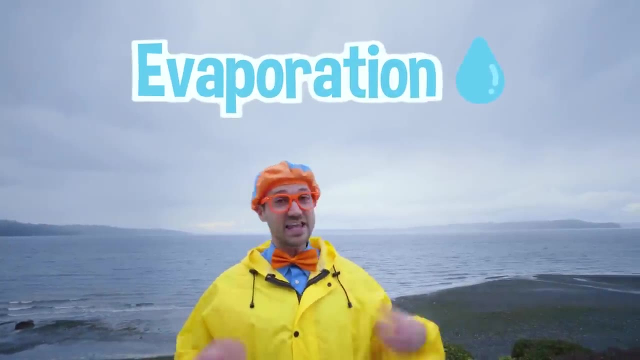 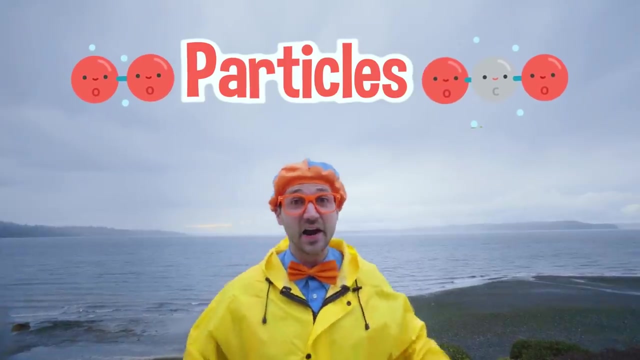 Yeah, Water is a liquid at this time and place, And then water goes- what's called event, And then water goes what's called event evaporation. Yeah, evaporation is when the water becomes these little tiny particles and goes up in the air. Yeah, it turns into a gas, goes up in the air and then. 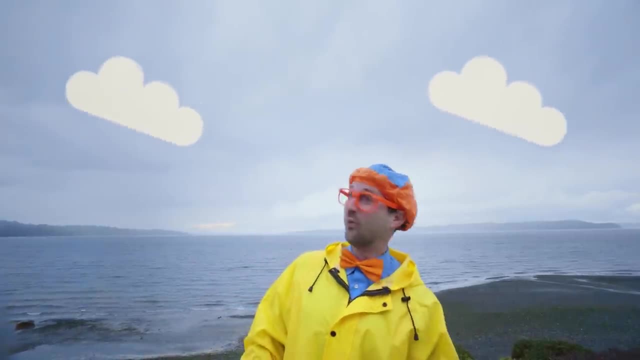 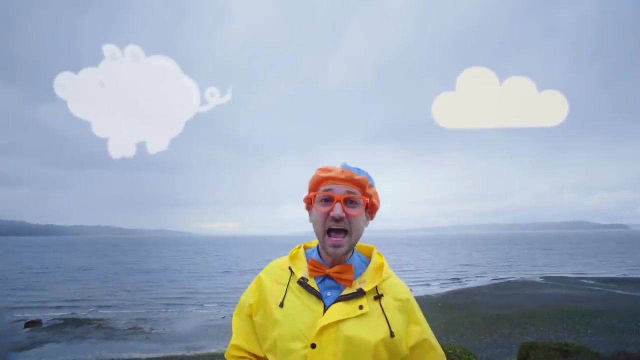 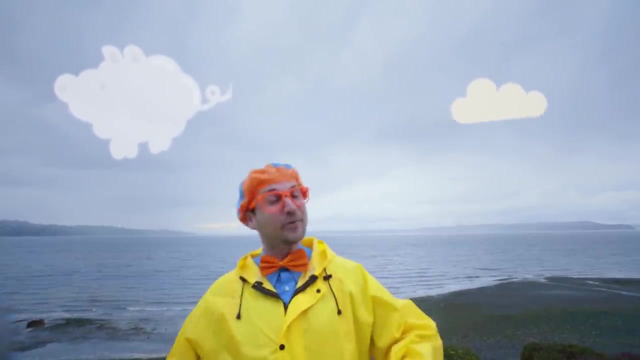 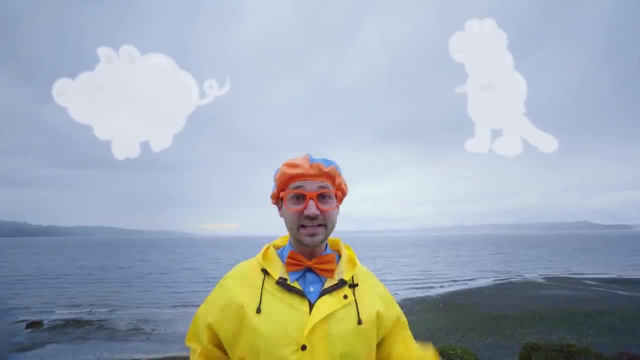 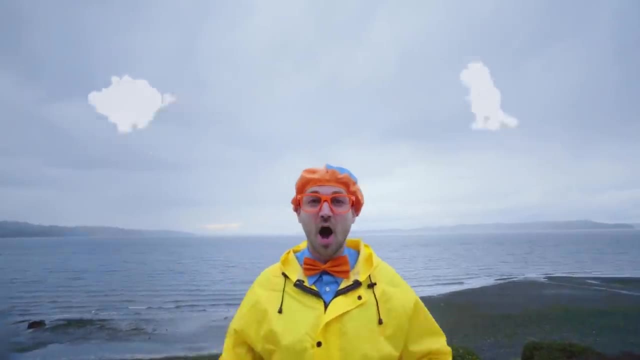 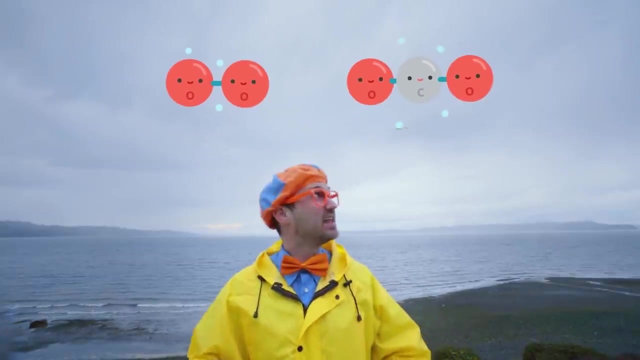 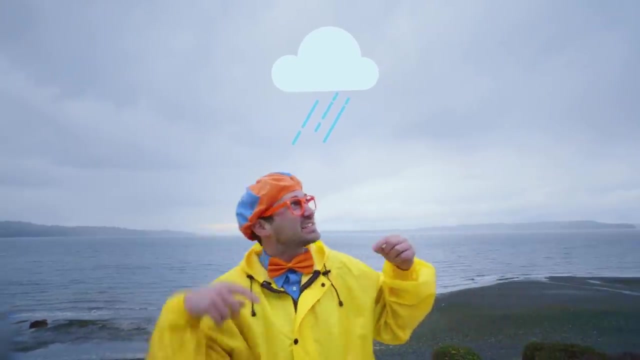 Look at that cloud. That cloud looks like a T-Rex: Rawr, rawr, Wow. And then all this gas water starts to come closer and closer and closer, Yeah, and those clouds start to form into liquid water again, Yeah, and then rain starts to fall. 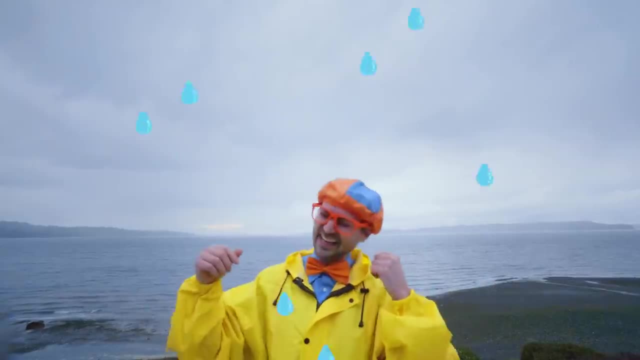 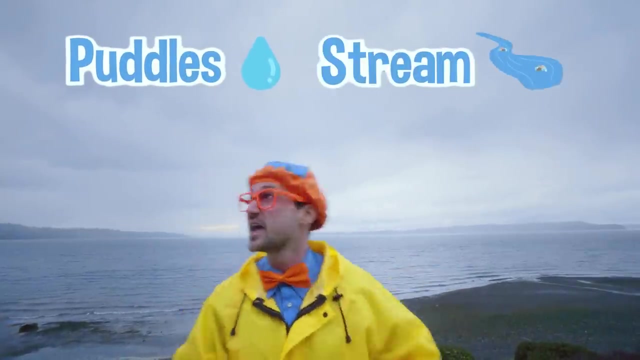 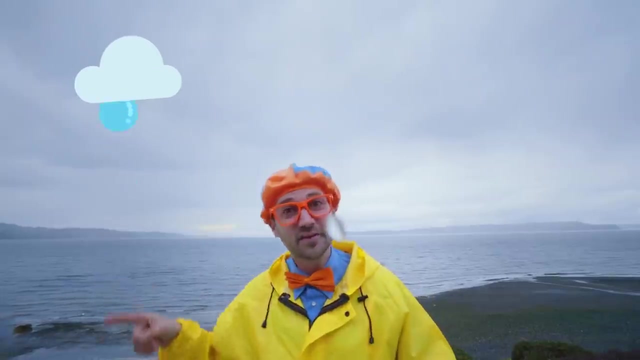 Woo, Yeah, it's raining, Whoa. And then they create puddles and streams and ponds and the water goes back into the ocean again, And then the cycle goes over, and over, and again and again. Wow, that water cycle is so great. 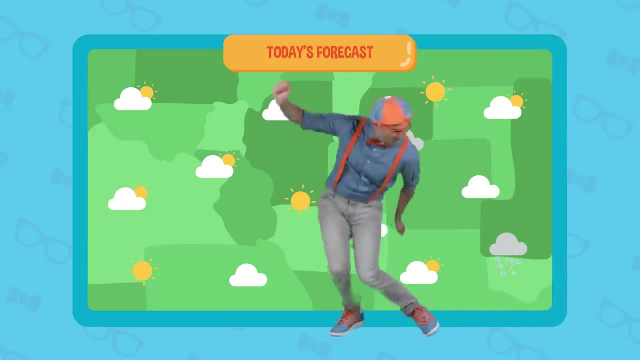 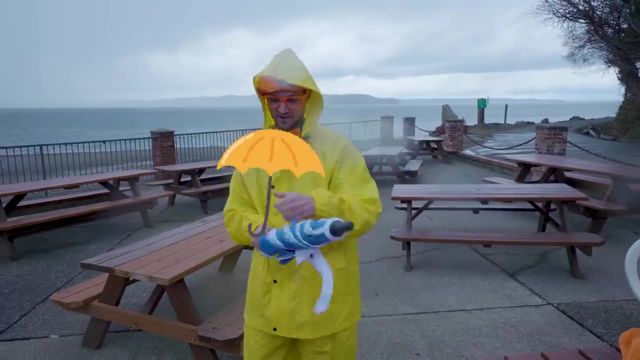 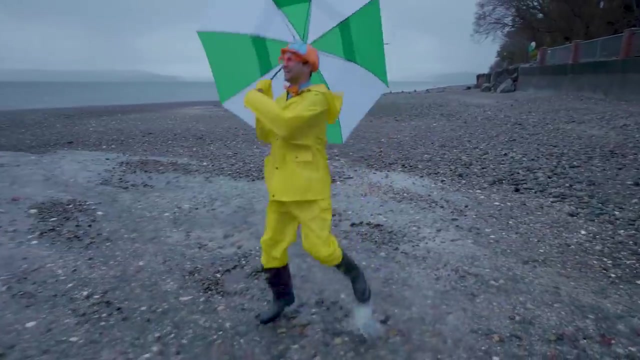 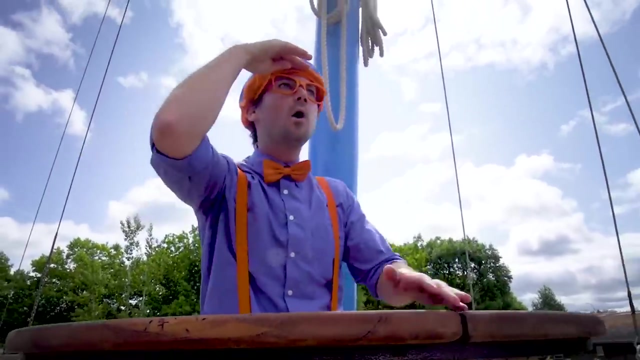 Woohoo, Today's weather forecast: Sunny skies in the morning, Followed by storms in the afternoon. Don't forget your umbrella. The morning looks nice: Lots of sunshine, Clouds of white and a bright blue sky. But the sky's turning gray. 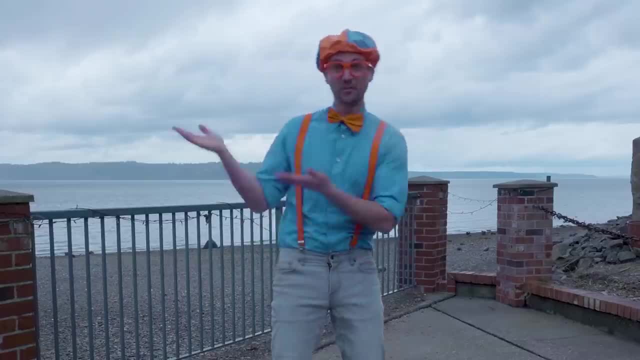 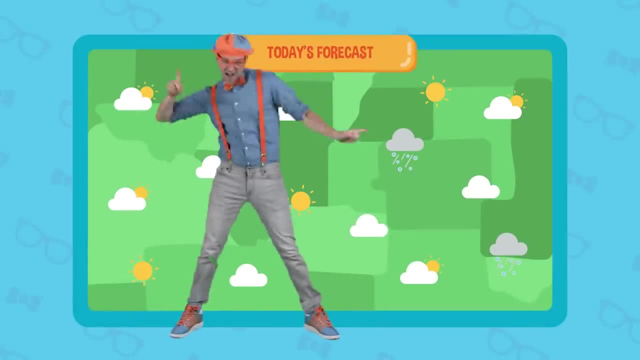 There's wind and some rain. It looks like it's going to be a stormy day. Weather weather- all kinds of weather, Like sunny, breezy, cloudy, warm, pleasant days. Weather weather- all kinds of weather. 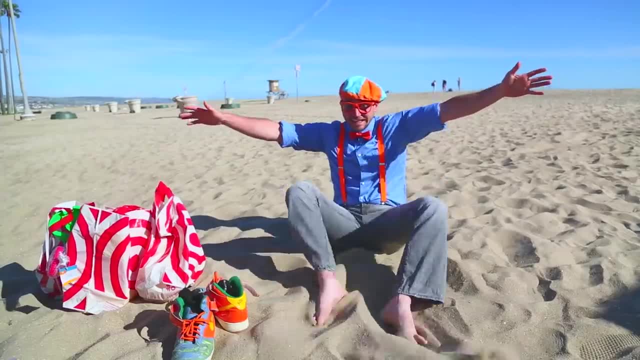 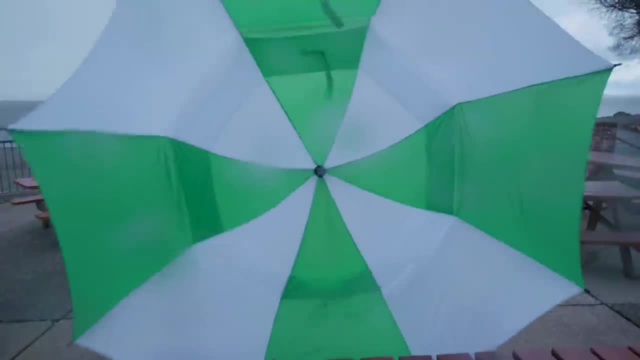 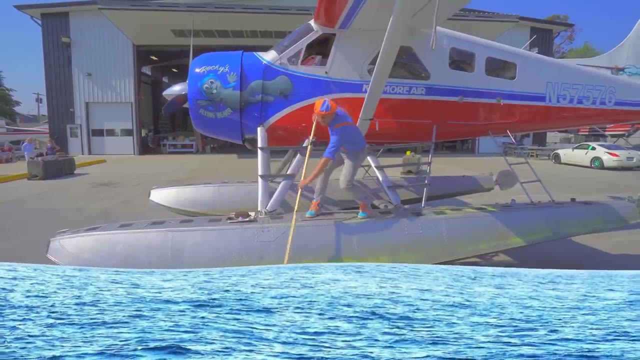 Like windy, rainy, stormy, hot, muggy days. A lightning bolt, That thundering sound. There's a storm coming any moment now. Tornadoes, hurricanes and floods, Hurricanes and floods. Sometimes weather can be dangerous. 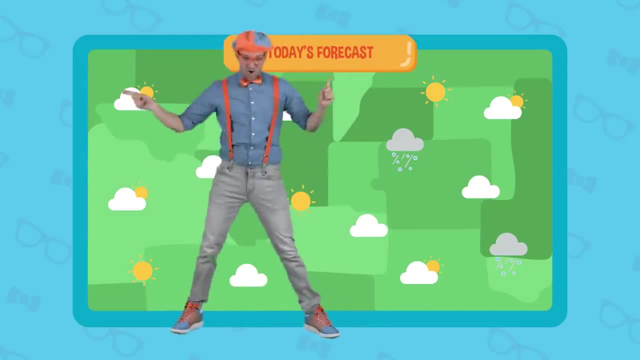 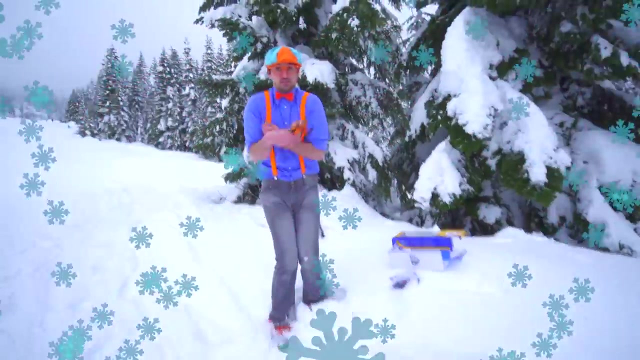 Weather weather: all kinds of weather Like sunny, breezy, cloudy, warm, pleasant days. Weather weather: all kinds of weather Like windy, rainy, stormy, hot, muggy days And when it's really really cold. 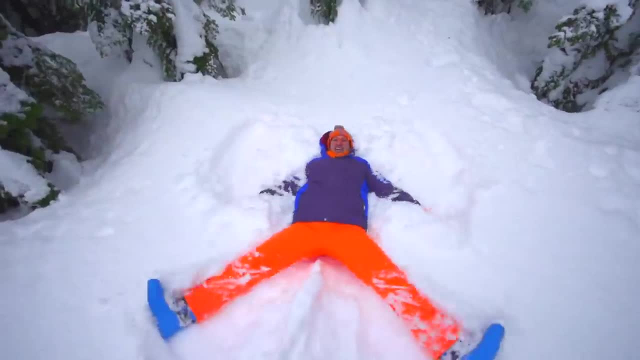 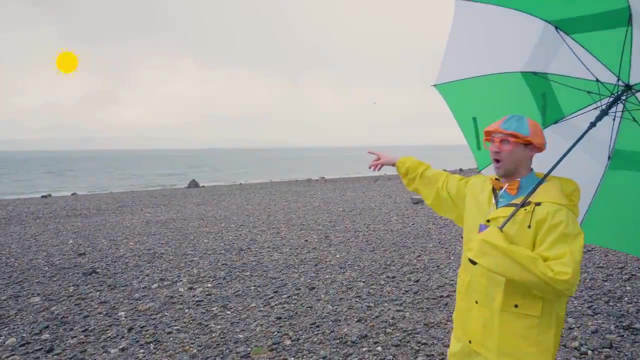 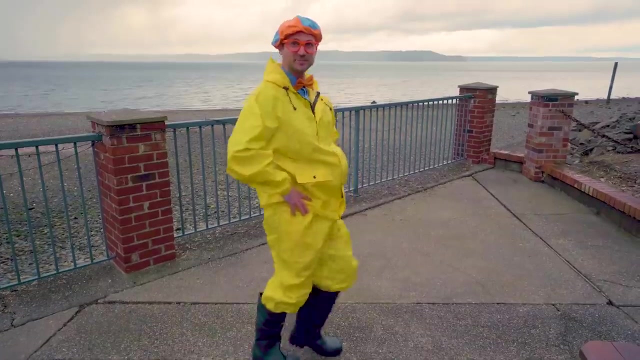 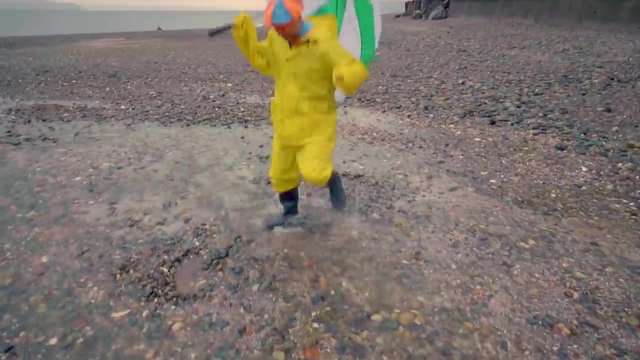 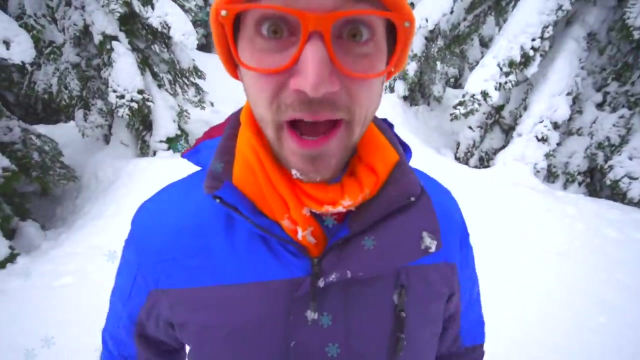 snowflakes will fall from the sky, Everything goes quiet and everything is covered in white. Hey, The rain has stopped and the sun's shining again. Weather weather- all kinds of weather Like snowy, icy, blizzard, cold, frigid days. 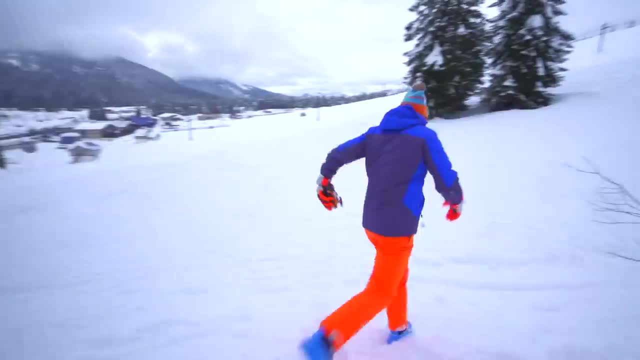 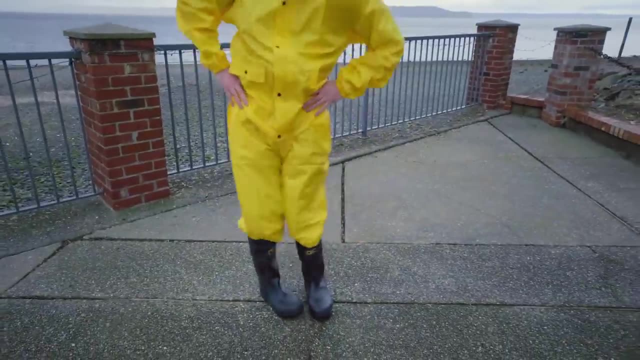 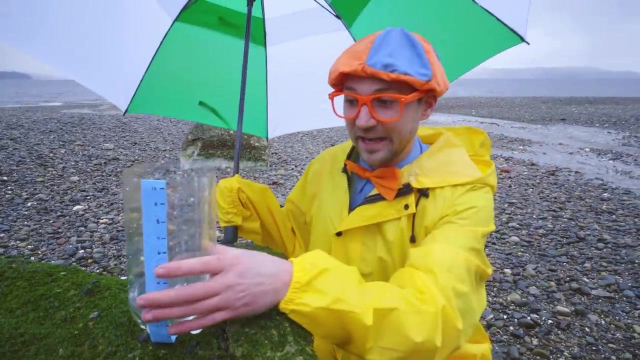 Weather, weather, all kinds of weather. Well, this is the end of this video, But if you want to watch more of my videos, all you have to do is search for my name. Will you spell my name with me, Ready? 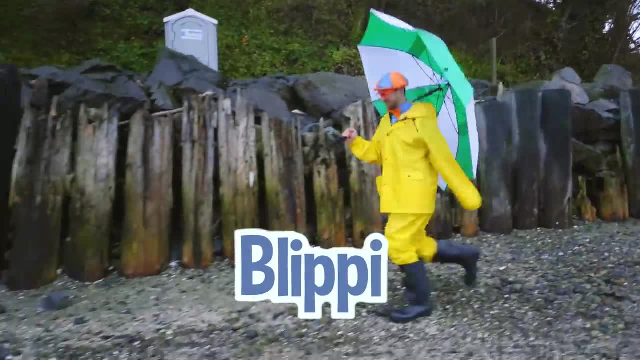 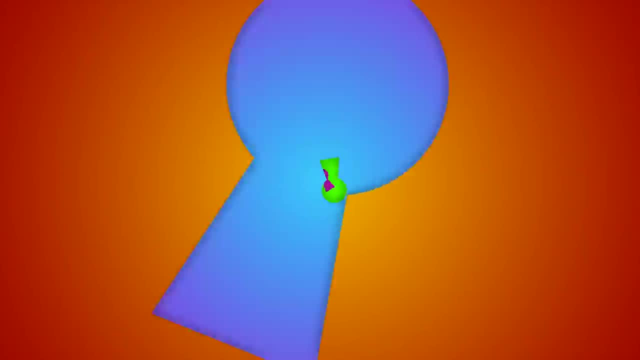 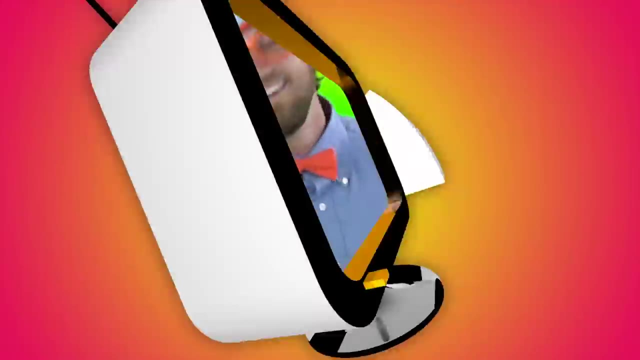 B-L-I-P-P-I- Blippi. Good job, Alright, see you later. Buh-bye, Blippi. come on everyone, let's make money fun, Blippi, Blippi. So much to learn about. it'll make you want to shout. Blippi. 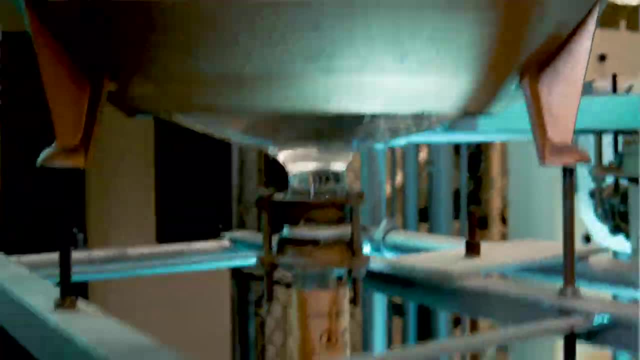 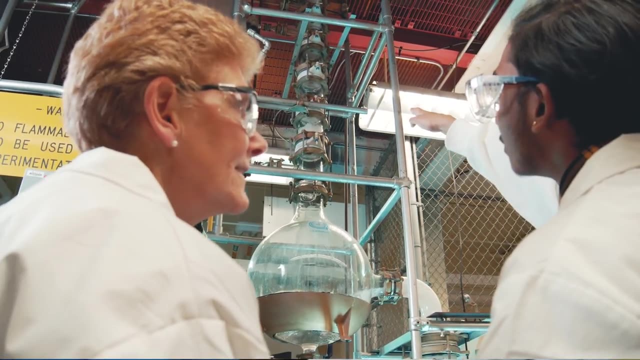 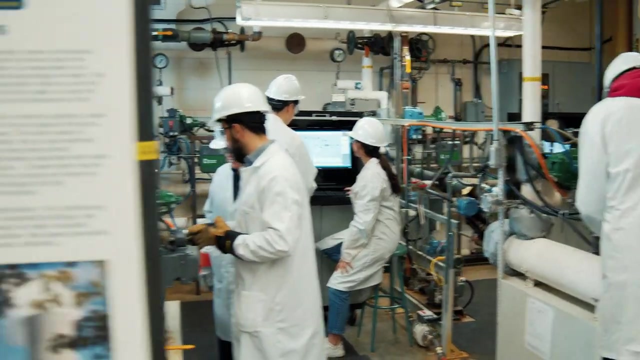 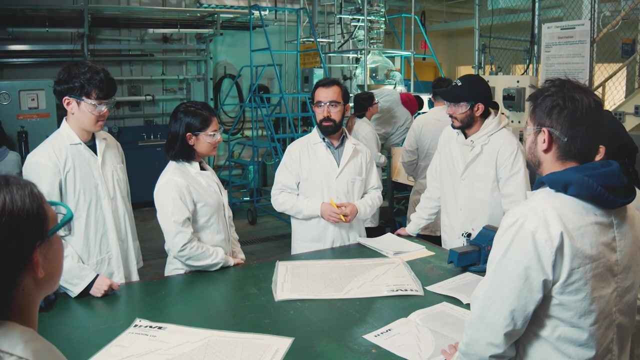 Well, I was interested in this program because I'm really passionate about the environment and climate change. I found BCIT and they had the chemical environmental technology program and once I went through the course outline I was like, yeah, this is a program for me. Our chemical and environmental technology program is basically a two. 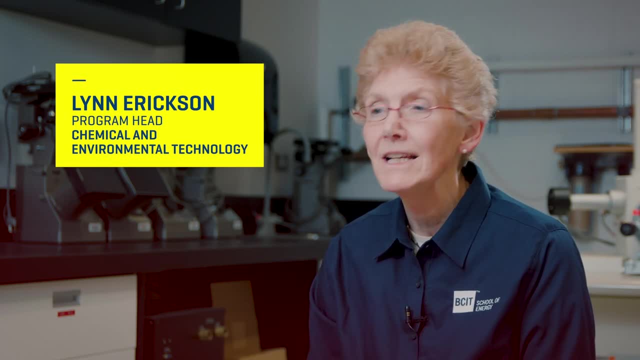 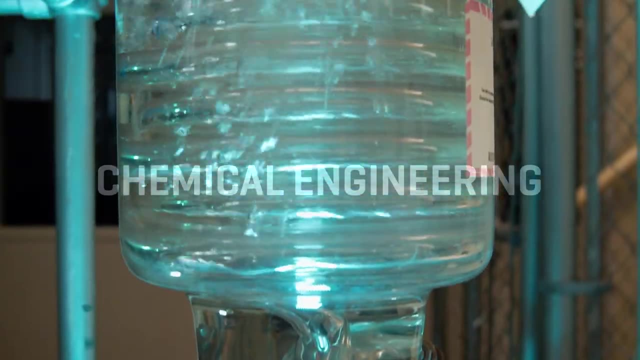 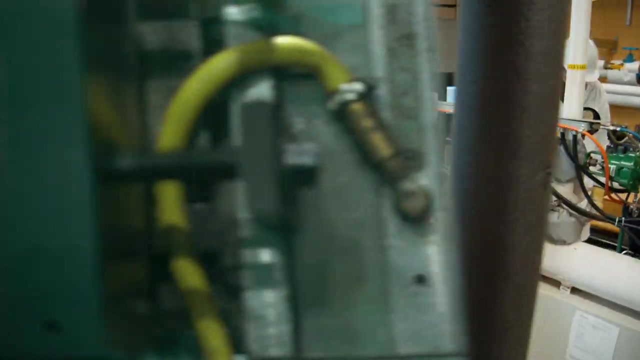 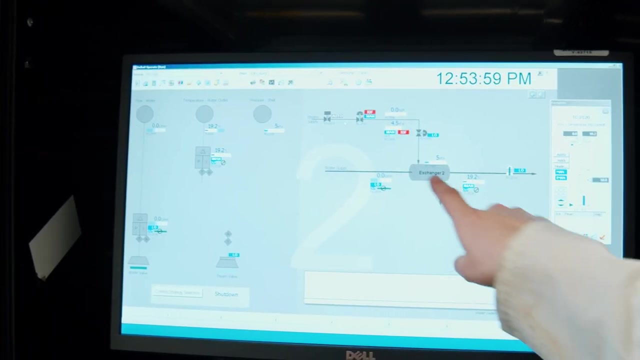 year diploma program where students learn the the latest and analytical techniques, chemical techniques together with environmental science and chemical engineering, mineral processing materials technology and many other techniques. We also do simulations and do computer analysis. so they're actually learning how the flow charts and trying to simulate the whole process. because if 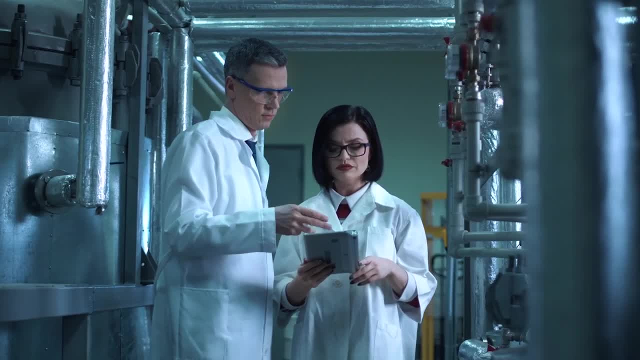 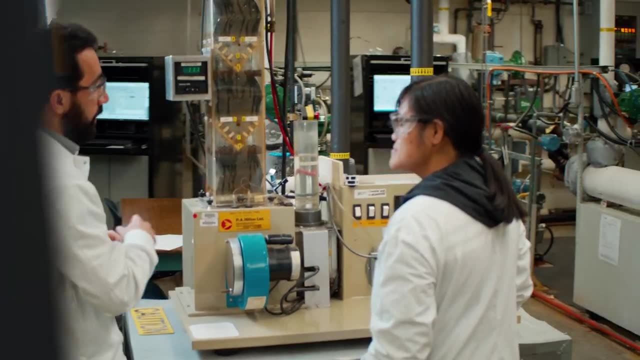 you imagine, in a chemical process plant you may have a number of the people, piece of equipment we have in our lab, but they're all connected together to create a process, to create a product. Jobs they would get when they're graduate. they could be working with green. 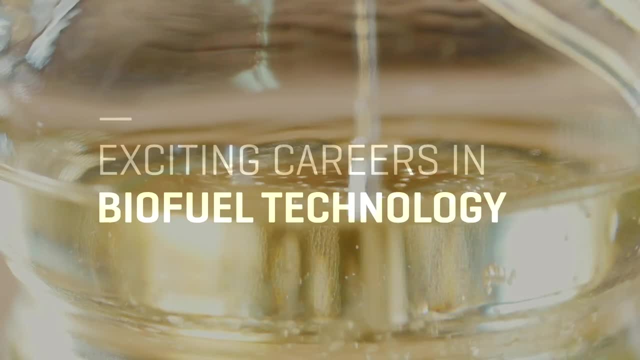 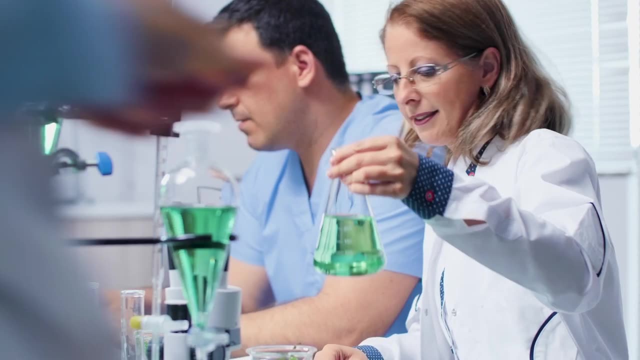 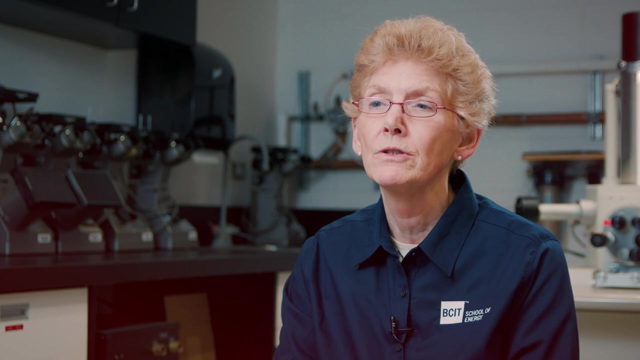 industries like batteries, fuel cells, biofuels, biomass. A lot of the newest industries are hiring our students. basically, Some of our people go straight out of this program into either a Bachelor- they can do a Bachelor of Chemical Engineering. we have people do it going into. 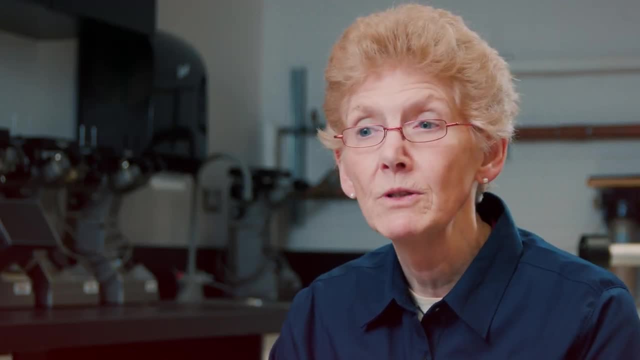 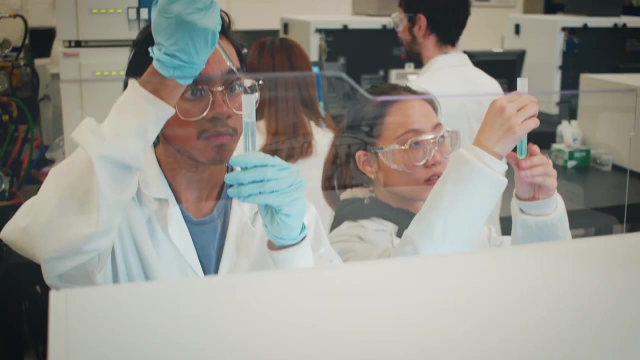 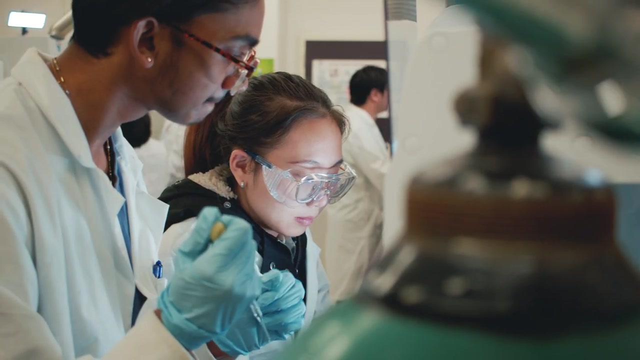 environmental. it opens up a lot of possibilities. You can go out and work, save some money and then go back to school if you want. Well, through this program I've had a lot of time doing different research projects. It's given me a skill set. I need to be able to analyze to be able to 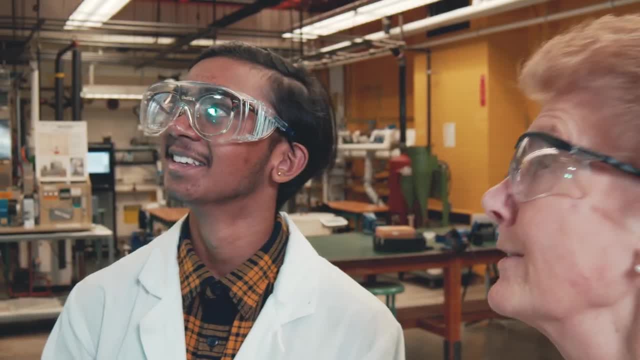 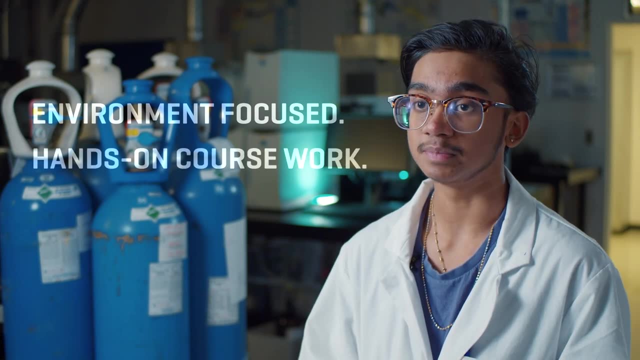 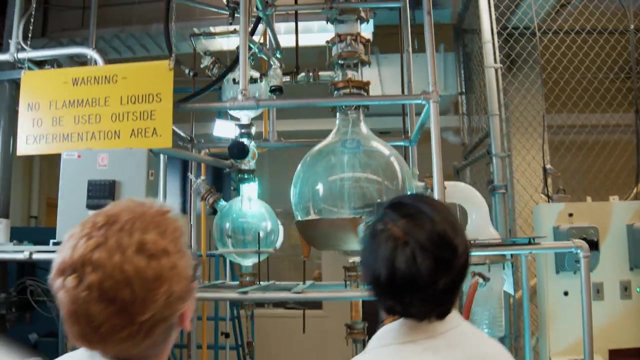 research and the mentors that you need to be able to do this. If you're passionate about the environment, you like hands-on work and you want to be in a job related to this, then I definitely recommend this program for you, because you're gonna get all that.